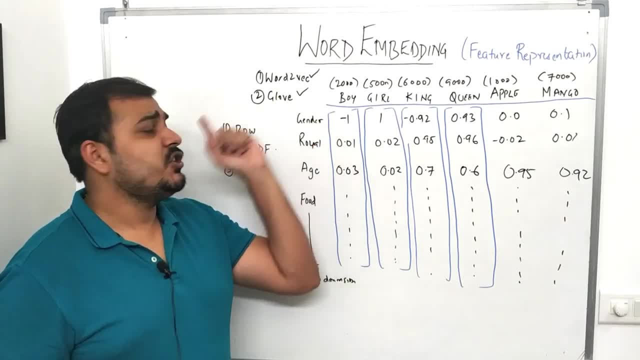 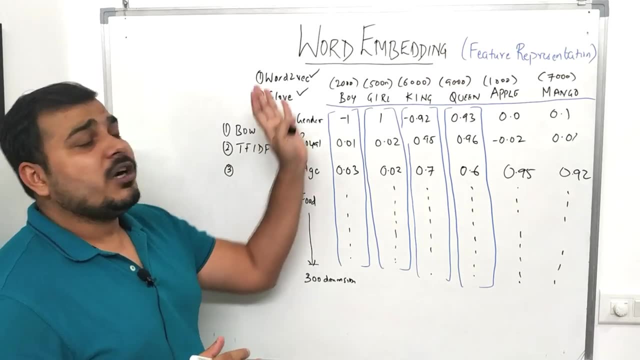 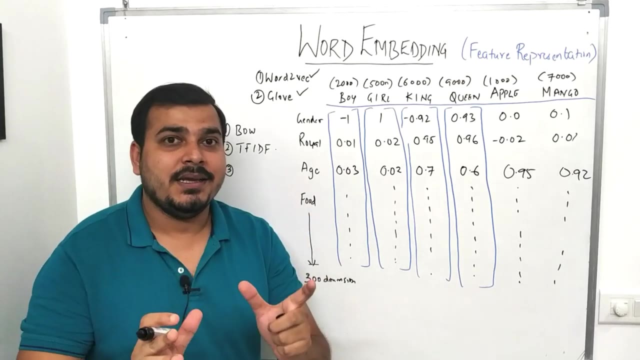 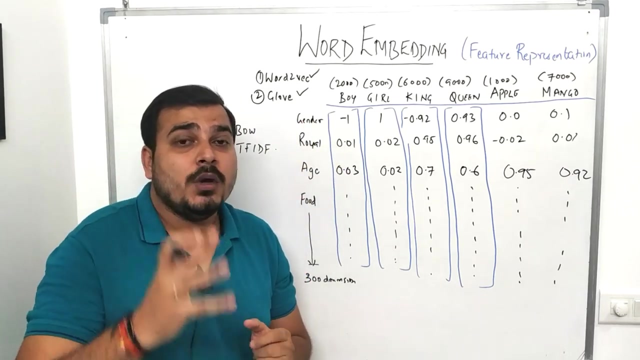 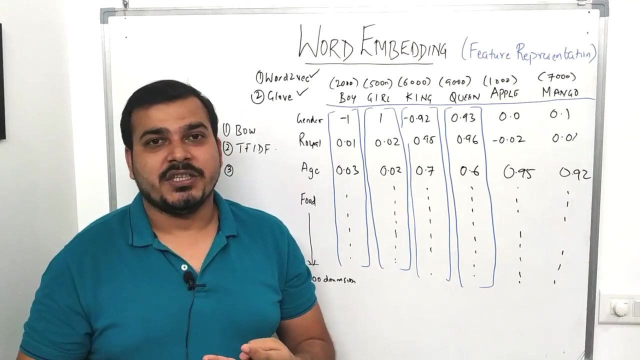 I will be covering both these in NLP playlist. I have already uploaded the explanation regarding word2vec, right, and then we will also be taking with will be able to generalize this words to do any kind of predictions or to do any kind of sentence generation and many more things so that we'll try to discuss. so let's, let's go ahead and 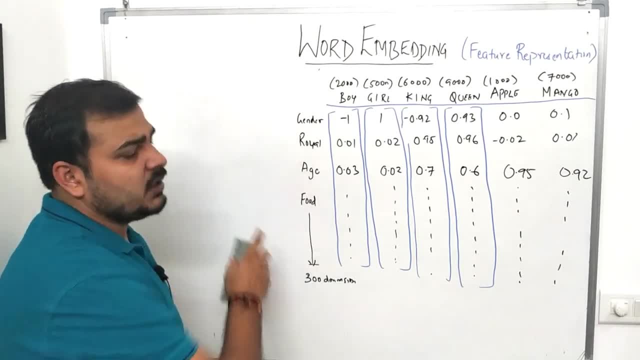 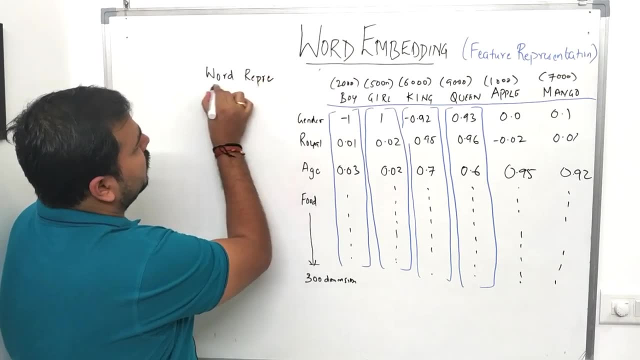 try to first of all understand some important or basic terms with respect to word representation. so i'm just going to write over here as word representation. okay, now suppose in this word i have a dictionary which is having somewhere around 10 000 words. okay, so i'm having a. 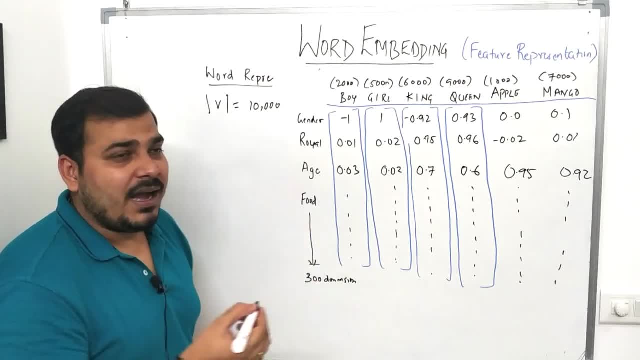 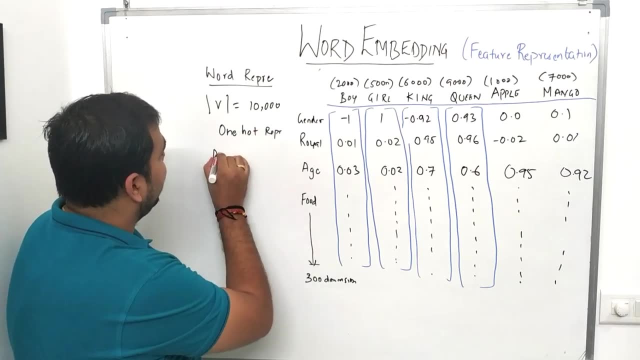 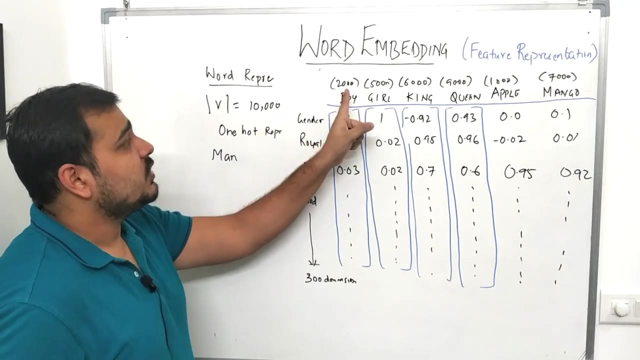 dictionary where i have 10 000 words. now, if you remember bag of words, i can also say it as one hot representation. okay, suppose i take a word like man and this man is actually present, you know, in this particular dictionary of words at the 5000 location, or suppose i can say it as. 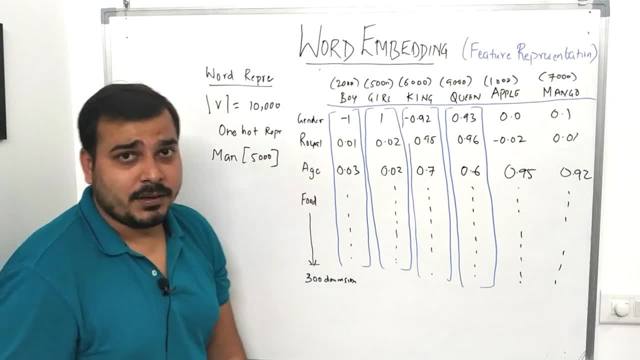 it is present in the5000 location. suppose i'm just taking an example. now, if i want to convert this man into a vector in the form of one hot representation, what i can do is that i can take 12, 10,000 word vector representation like this. all the other words will become zero, only this man word. 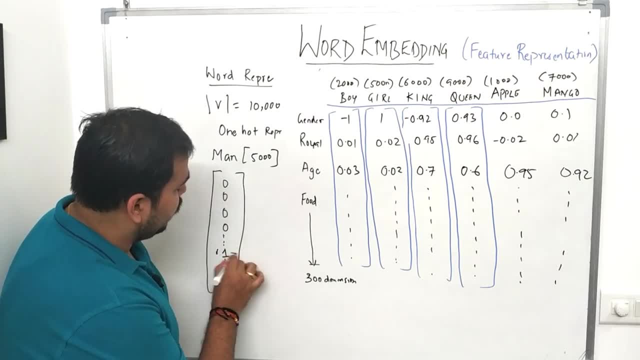 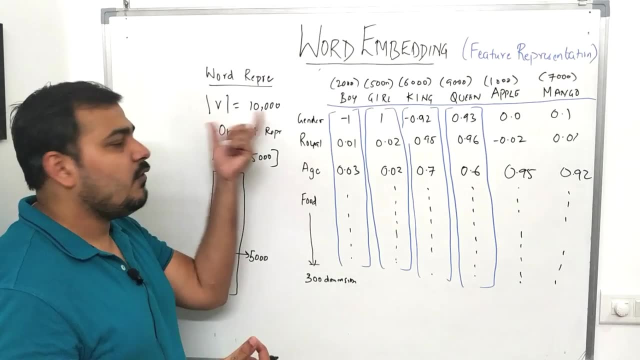 here will be becoming one and remaining all will be zero. this one will be the index of 5000, right? so this is the index of the dictionary, and remember, in dictionary you have all the words in sorted order with the index, right? so suppose this is present in the 5000 index now? similarly, 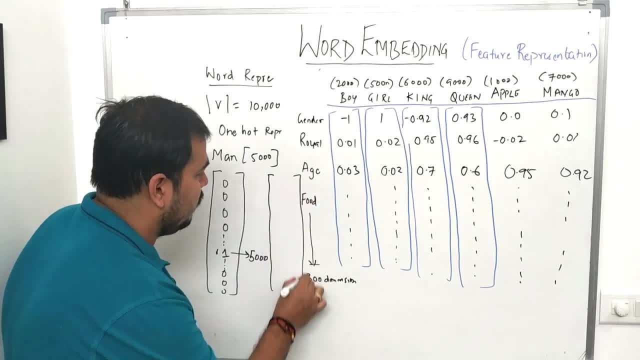 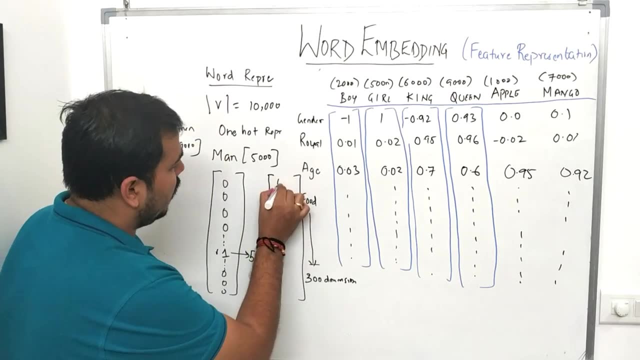 suppose i have one more word like human. okay, so suppose i have one more word like human. now this woman is present in 9000 index, right? so how will be this vector representation? it will be somewhere like this, and at the 1000 location i'll be having a one, right? so this? 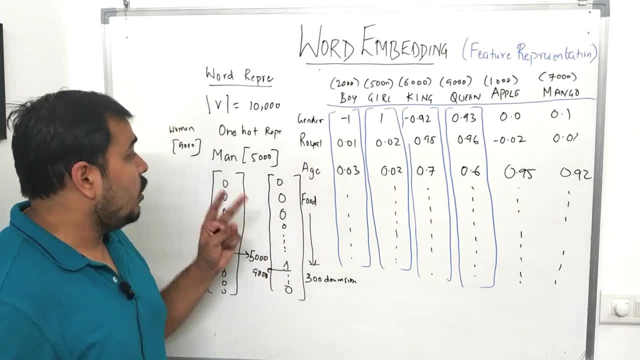 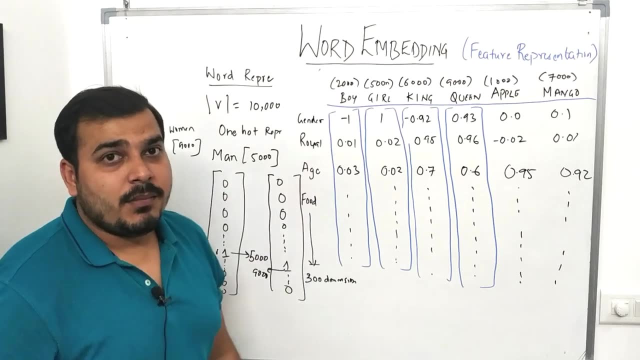 will be my 1000 location, 9000 location, sorry. so now you can understand that with the help of one hot representation we can actually convert this word into this kind of vectors. remember, in bag of words, we are actually trying to convert in a different way: in tf, idf, we are trying to convert. 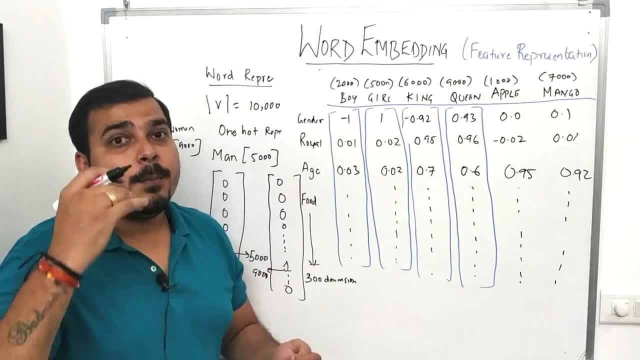 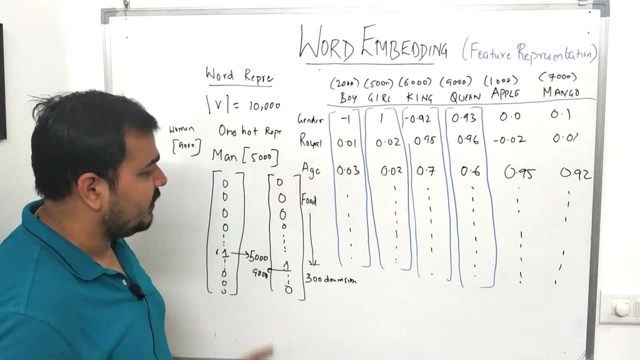 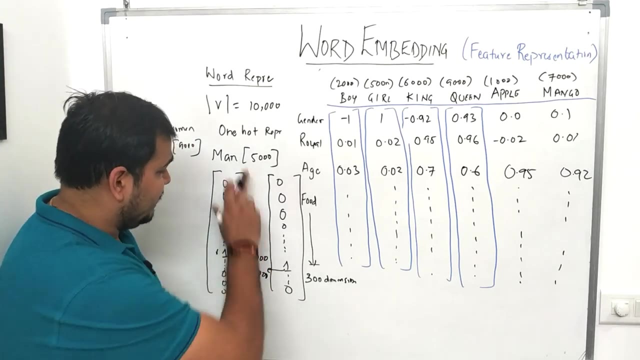 in a different way, which again had some disadvantages, but the efficient way to do it is by using word embedding. now, before understanding word embedding, i'm just showing you an example of one hot representation. so this is my man representation, vectors representation, and this is my human vector representation. now understand one thing, guys: this, this size. 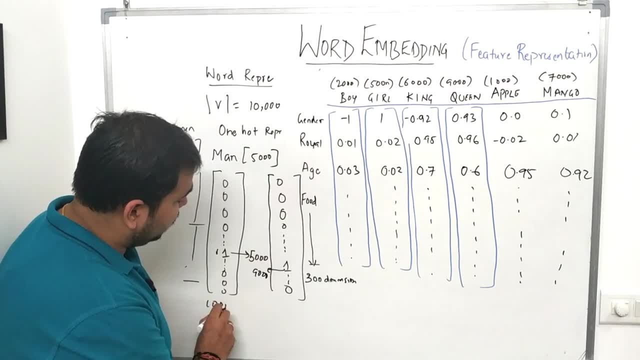 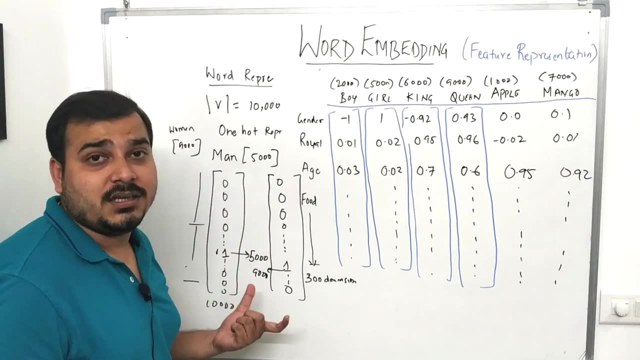 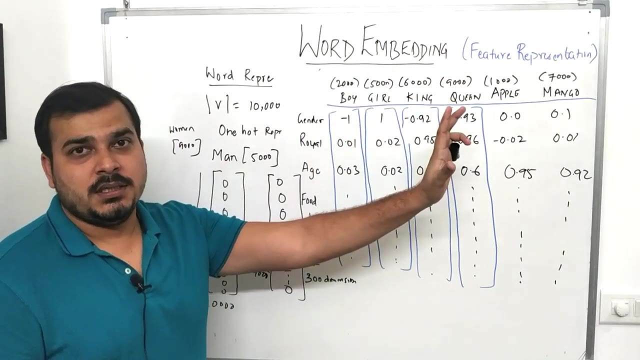 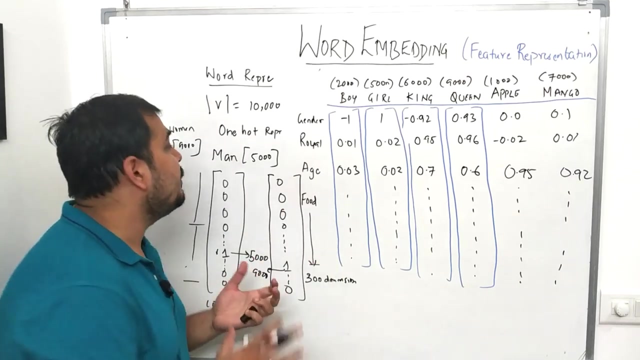 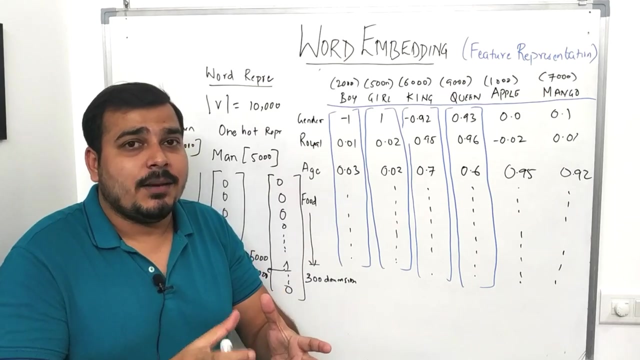 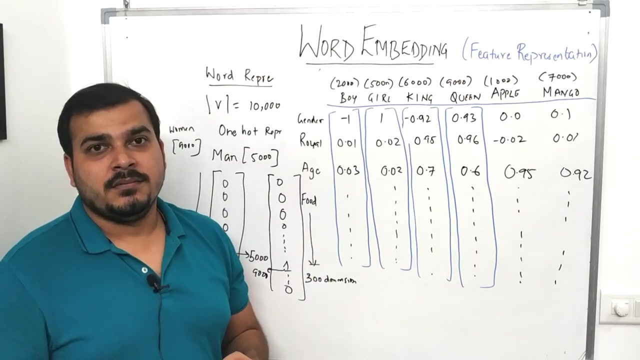 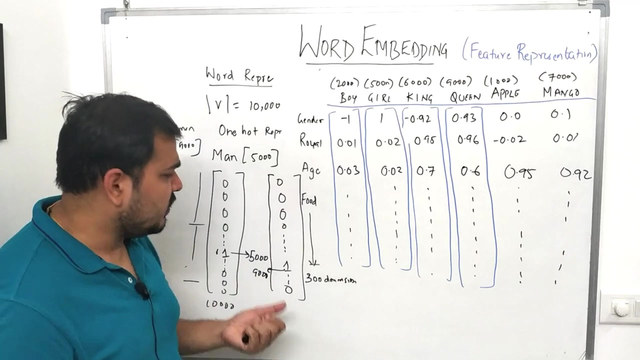 this whole size. right, it is somewhere around ten thousand dimensions, right, ten thousand words are there and we are actually converting this man into ten thousand dimensions or ten thousand vectors, right? so this is the vector representation and this is a very sparse matrix. Similarly, if I have many, many words, right, all the representation will be in this form only, right, where I'll be having zeros and there will be one index which will be having one. Now, what is the main problem with this particular representation? try to understand this. Okay, now, when my machine learning algorithm is getting applied, or a deep learning algorithm which is getting applied, it is very difficult, you know, it is very difficult to generalize these vectors. Okay, I cannot understand, like, if I want to find out the similar words, right, it is very, very difficult to understand from this because 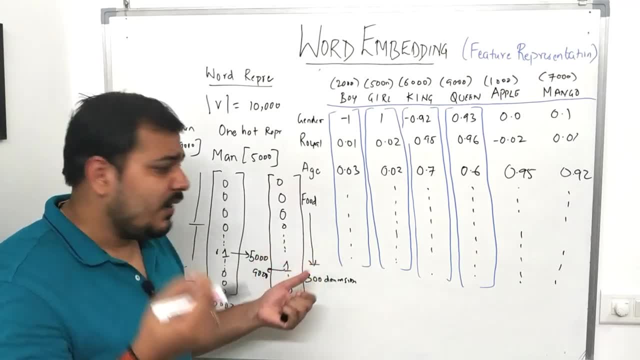 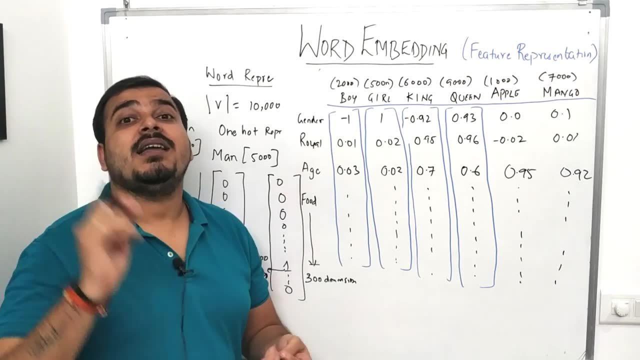 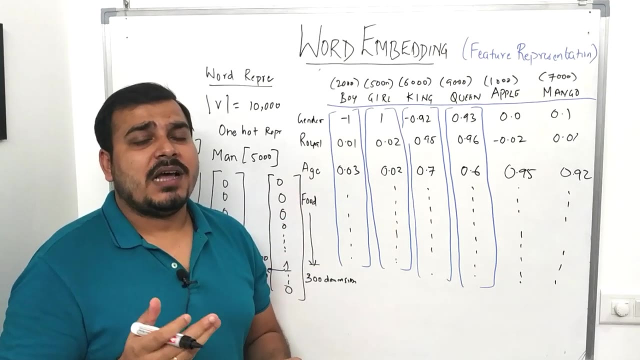 some or the other index in every word. you know that only one vector will be one and remaining all vectors will be zero. So definitely similarity of the words also cannot be found out. there is no much semantic information of the words also. So if I say semantic information, that basically I want to find out similar words. Let me take a very good example. Suppose I say that I want to eat a pineapple cake. Okay, the second word is that I want to eat an apple cake. Now suppose I have in my training data set where I have the sentence that I want to eat an apple cake. 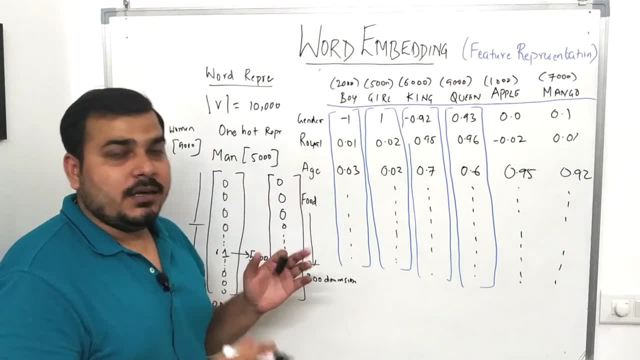 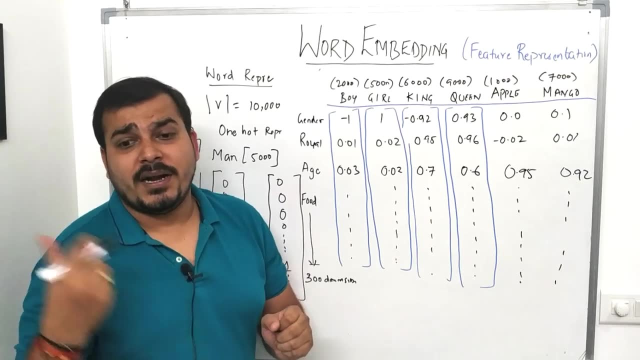 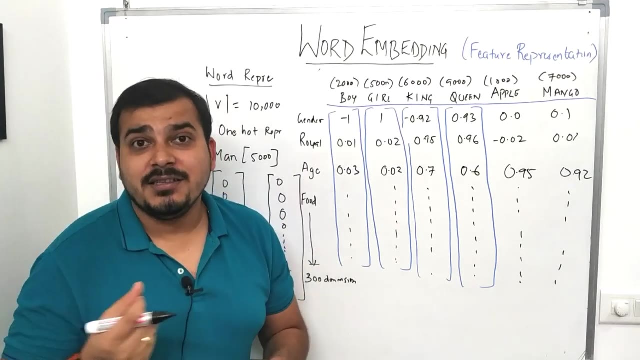 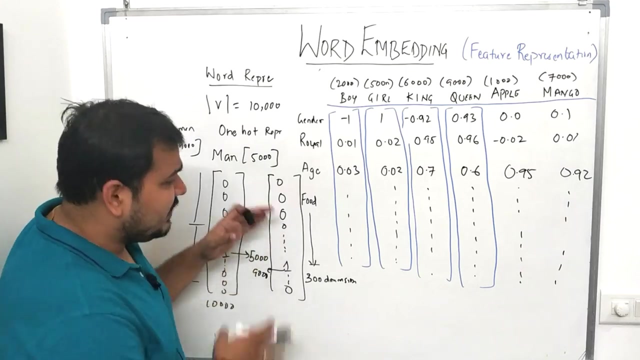 I want to eat a pineapple cake Right now. pineapple and apple, if I, if I see, with respect to this representation, I cannot conclude that they both are similar. right, Both are similar. Now suppose if I want to predict what will be coming in front of apple, then it will not be able to find out, it will not be able to generate the sentence. that is just an example what I'm taking, Right? So this has a lot of disadvantages. You know it is sparse And you can see the size is very big. right, The size is around 10,000 vectors. just just imagine 10,000 vectors. 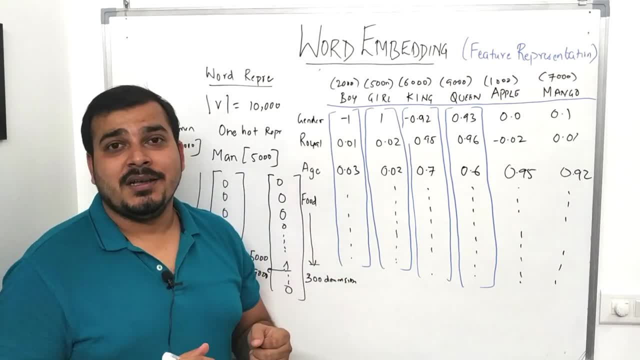 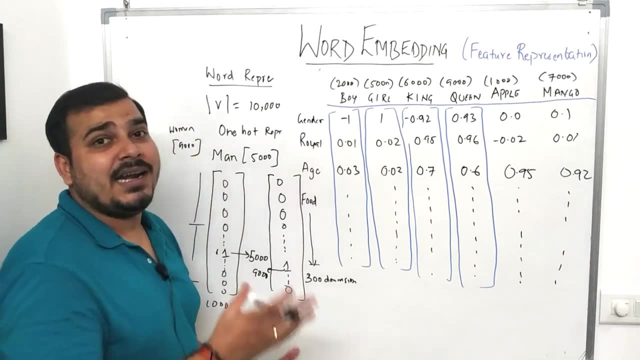 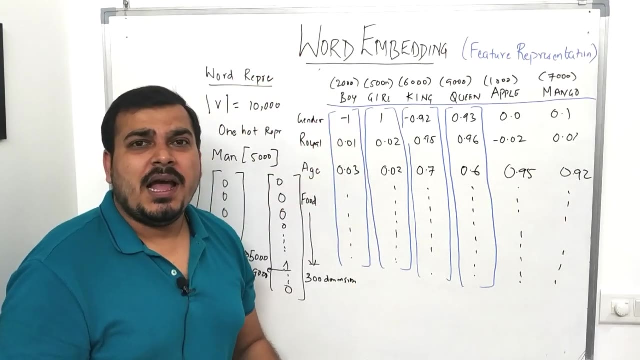 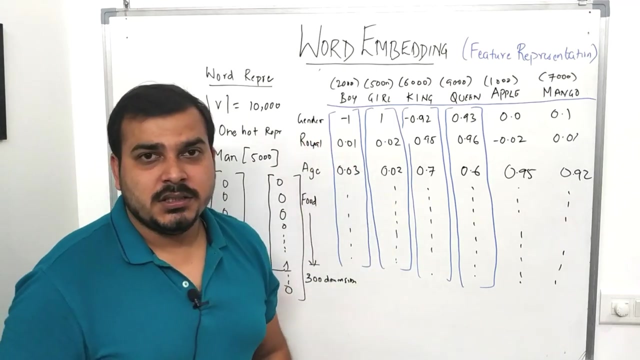 Sometimes, if you, it will be very difficult for you to execute right, The car, the model will not be able to also give you a very good results right. So you can understand that this is very, very high dimension and it is spot. it is having a sparse matrix. Sparse matrix basically means that you have so many number of zeros and you have less number of ones. Okay, so this is what a sparse matrix basically indicates. Now, in order to overcome this particular disadvantage, you know there's a concept that is something called as word embedding. Now, in word embedding, 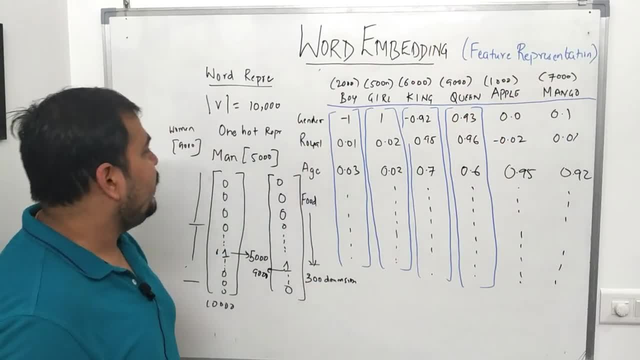 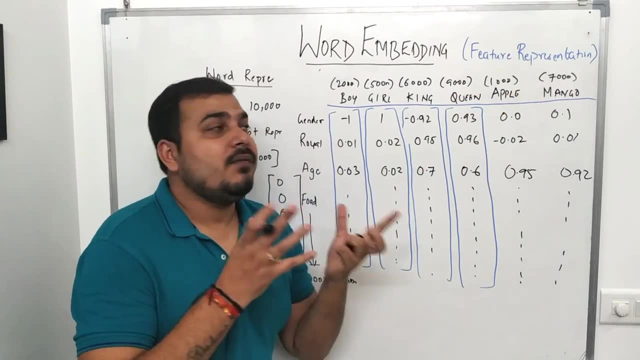 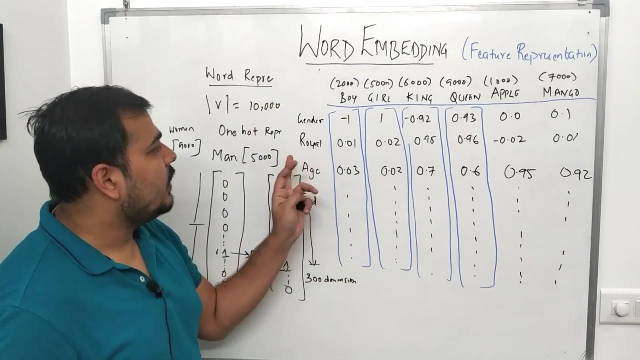 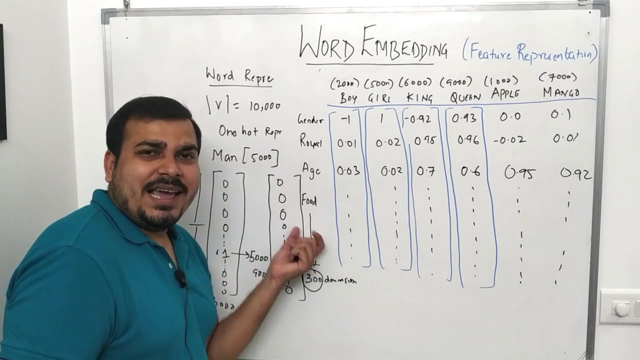 there is a concept of feature representation. Now what we do is that we take all this 10,000 words, or suppose, if I'm considering this words like boy, girl, king, queen, apple, mango- we will try to convert them into vectors based on some features. Now, what are the features over here? Suppose we have taken some features like gender, royal age, foot, blah, blah, blah, blah- somewhere around 300 features are there. Okay, so it can be any number of features, like action, you know, or I can say good, bad, something like that. Right, So those kind of features. 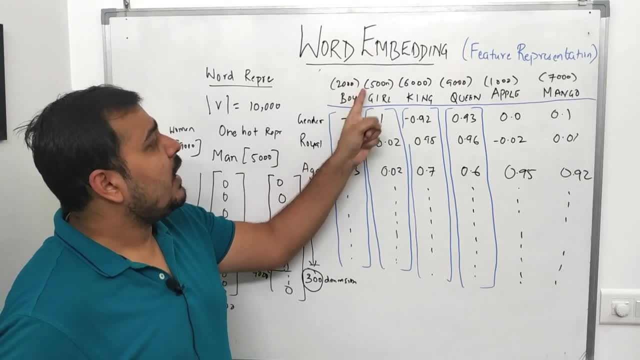 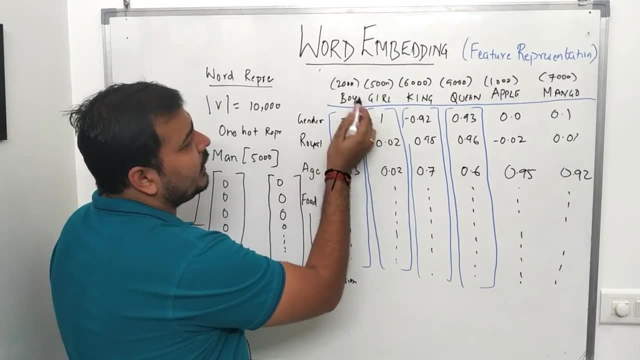 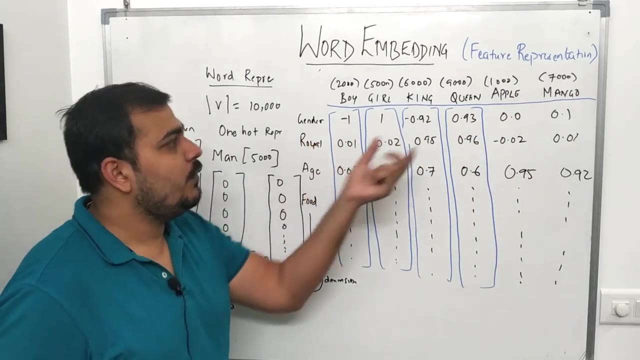 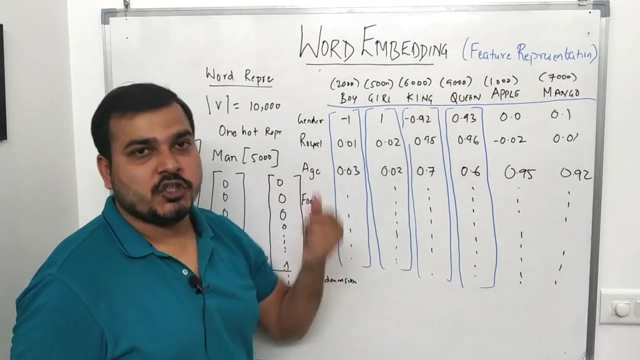 can be selected And based on this particular feature. whatever our words are, we'll try to convert that into vectors. Now how this particular feature looks like, understand. suppose this gender is now related to boy, girl, king and queen. it is not related to apple and mango. You can understand this right, Because gender is nowhere related to apple or mango. If I take fruit, fruit is an example which I can relate to apple and mango. At that time I cannot relate to this particular feature. Now suppose I have vectors like minus one, one for boy, girl. you know which is uniquely? 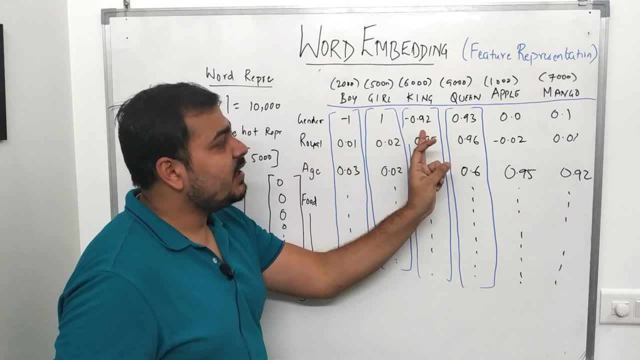 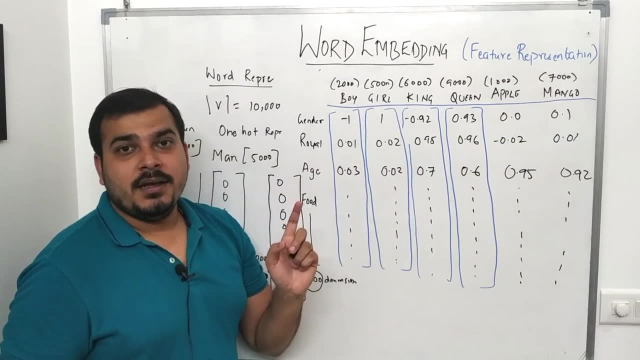 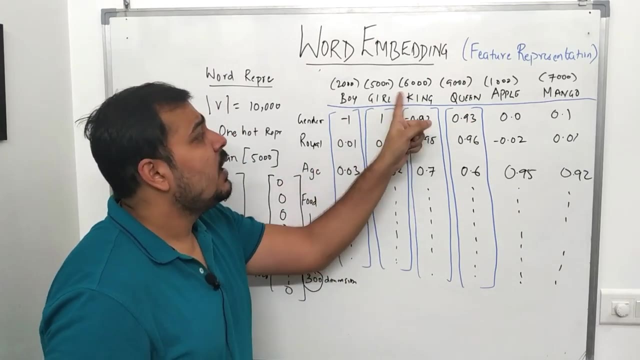 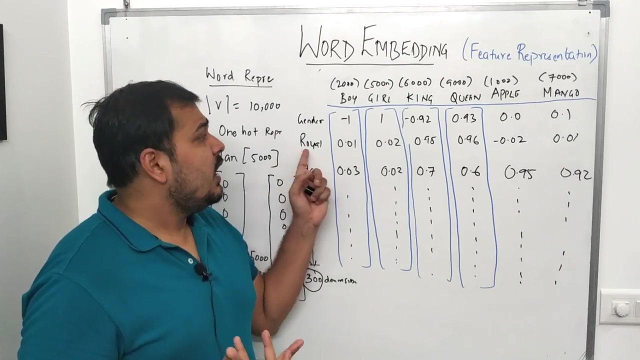 represented. You have king and queen, which is uniquely representing like minus 0.92, 0.93, right, But when I come to apple and mango, it is 0.0 and 0.1. Right Now, in this particular example, you can see that gender, we can see that, we can clearly see that, okay, there is a representation with respect to boy and girl, king and queen, right Now. suppose, if I go to royal- definitely if I, if I have a word, if I have a feature called as royal, if I want to relate, that I can only relate with king and queen. I cannot relate with some other features or some of the words over here. 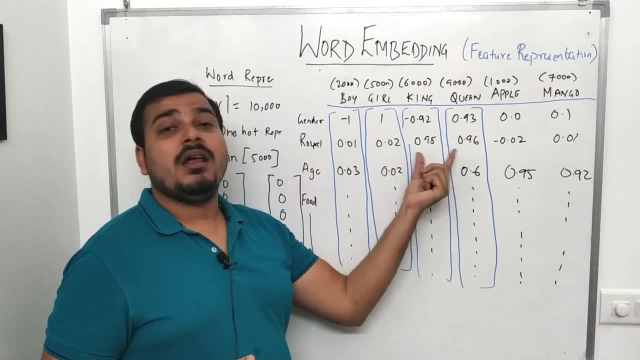 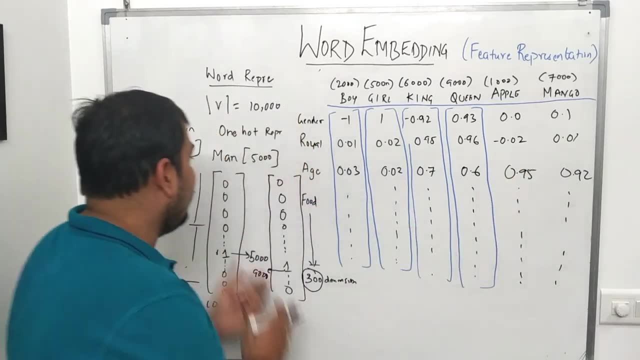 right. so at that time, these values will be little bit higher, and this will be similar also, since the value is very, very much near. this value is very, very much near. this value is very, very much near right. so, instead of making this one hot representation, what we focus on is that we 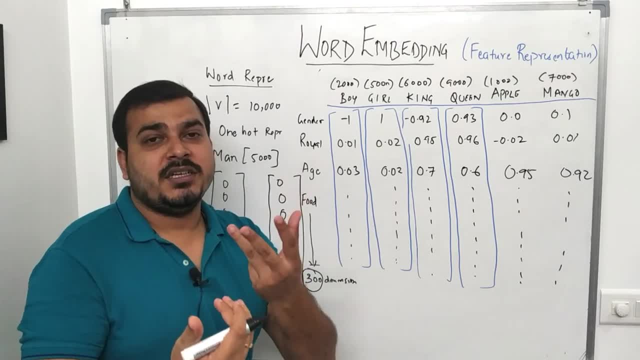 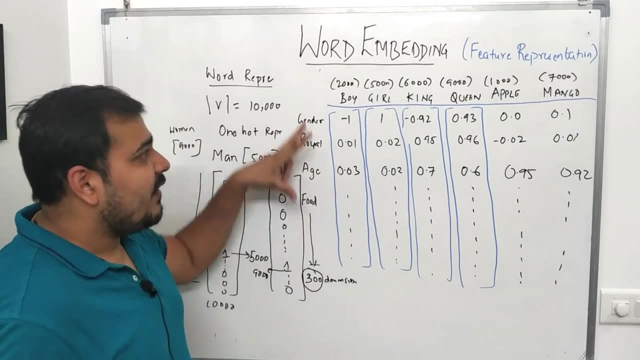 want to create this featurized representation. a featurized representation basically means that I'm taking this particular word. whatever word are there, I know the index number. based on this index, I will be, I'll be having some features, and that with with the help of this features. 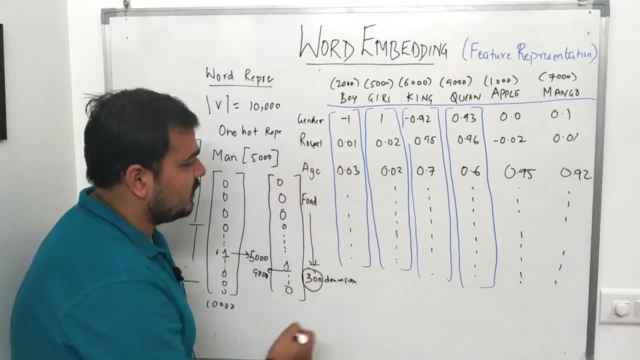 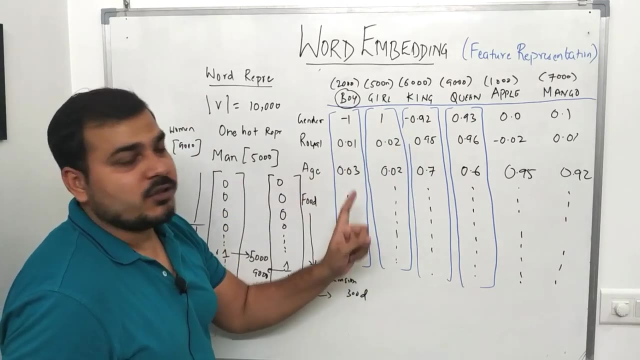 it will be represented in form of vectors. now what is the advantage of this? understand, guys? this all features, suppose I consider that- three to 300 dimensions, right? so this vector that is getting represented for this word is somewhere around 300 dimensions, right? similarly, for this word, I have 300 dimension, so this word, I have 300 dimension. so here I told, in one hot representation. 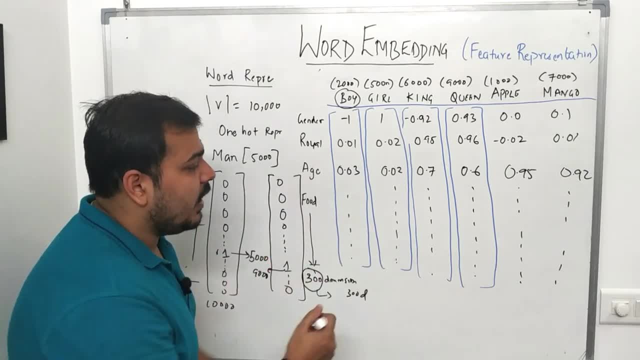 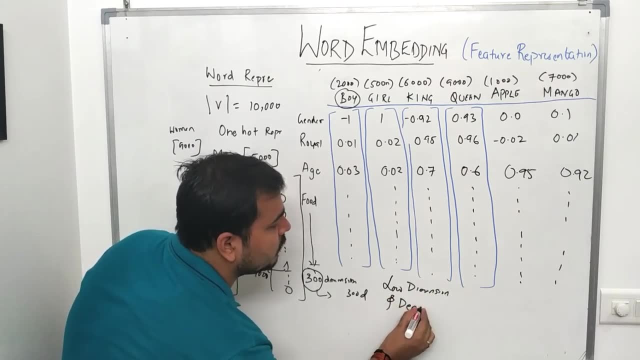 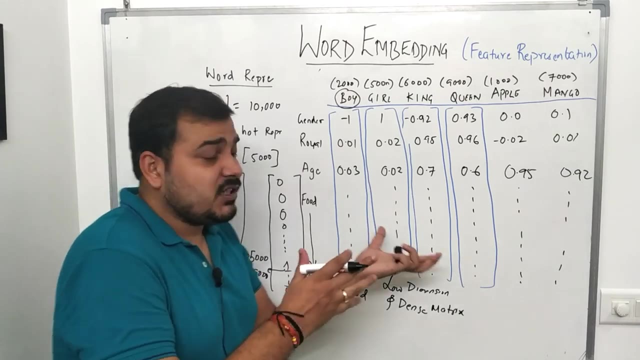 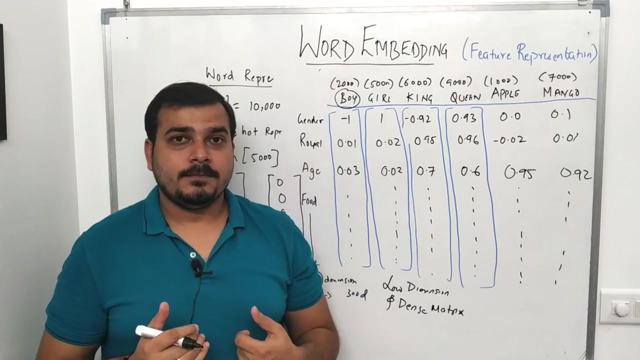 we have a higher dimension and sparse matrix. over here we have lower dimension and dense matrix. I can say it as dense matrix right now when I have this. okay, it is very much important now. what is the usefulness of this, guys? I I made a video regarding cosine similarity. okay, 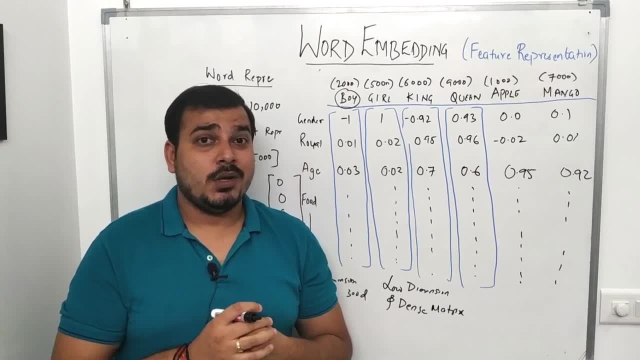 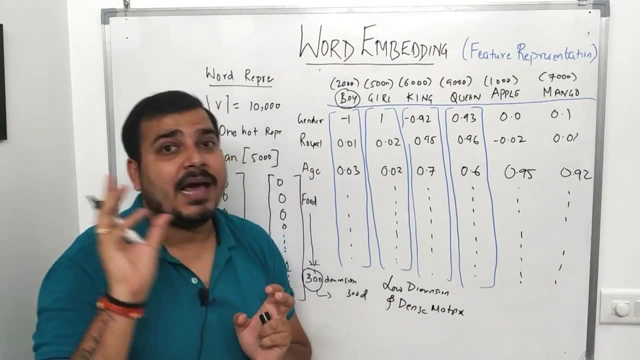 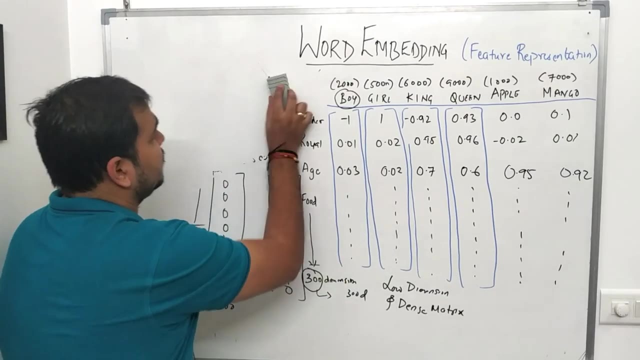 I made a video regarding cosine similarity in my machine learning playlist. you can go and check that particular video. that will actually help you to find out the similarity between two vectors. it will help you to find out the similarity between two vectors. now let's take this particular example. okay, suppose I'm just going to rub this so that you'll be able to understand. 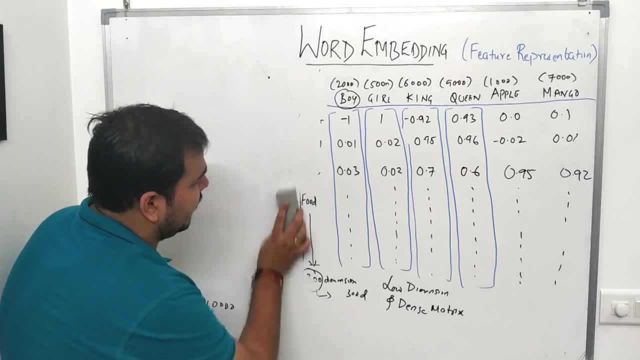 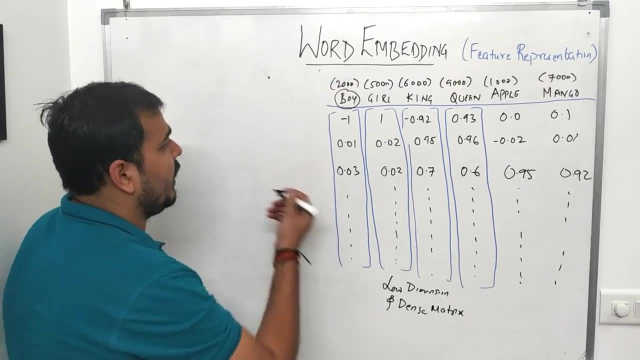 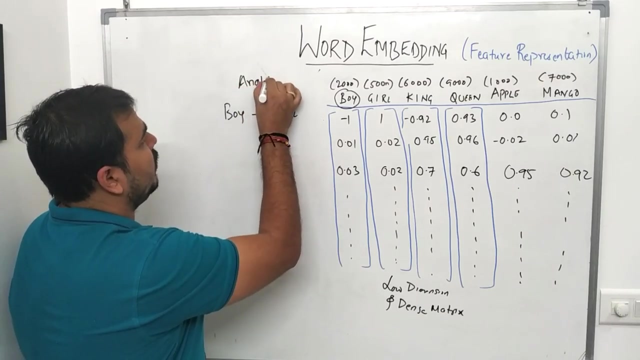 it properly. oops, sorry, I rubbed this part also, but I hope you have understood this. if not, you can actually refer. just going a little bit back, okay now, if I have a scenario where I say boy tends to girl, suppose I want to find out the analogy, analogy: okay, boy tends to girl. then 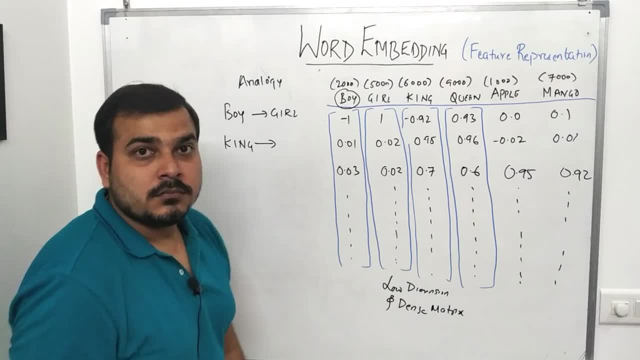 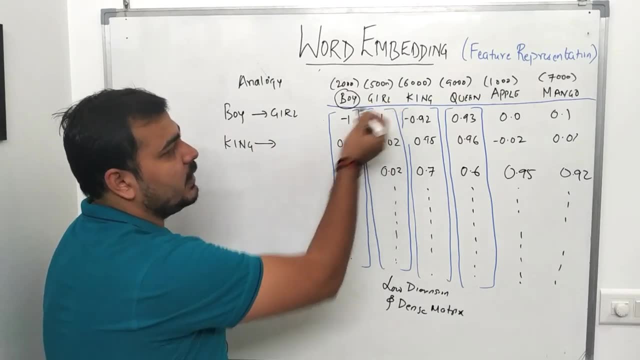 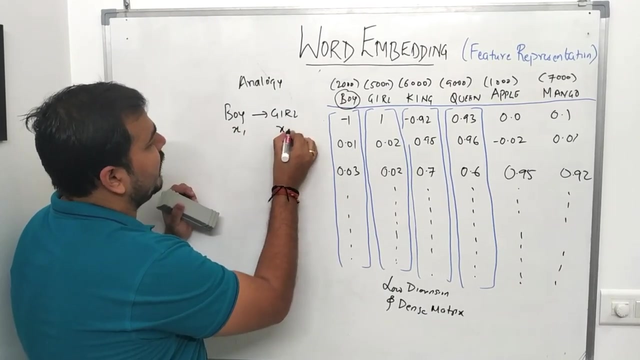 what? what do I say? what will King refer to? now? how this thing is going to work is I'm going to compute it. just understand this now, boy and girl. I know the vectors is over here and here. now, what I can do, suppose I consider that boy and girl vector. I'll consider this as my X 1. this is my. 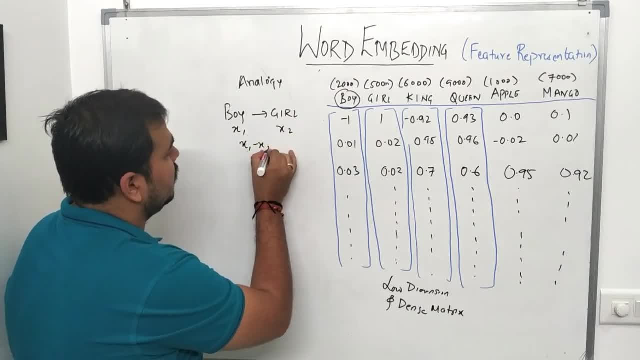 X 2. now if I do X 1 minus X 2, that basically means I am subtracting this vector with this vector, right? so I will be getting somewhere like minus 2. then all the values will be remaining zeros, right? in this particular case, you can see, it will be zero right now. if I do this, I'm going to 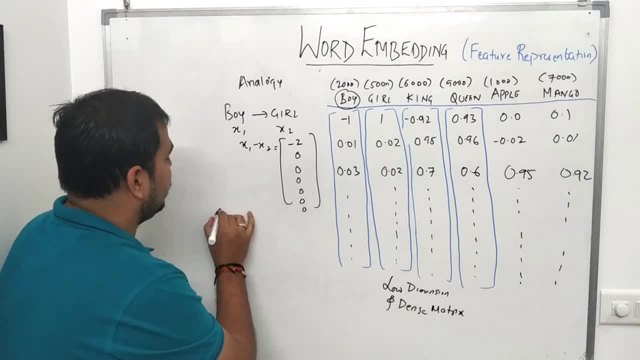 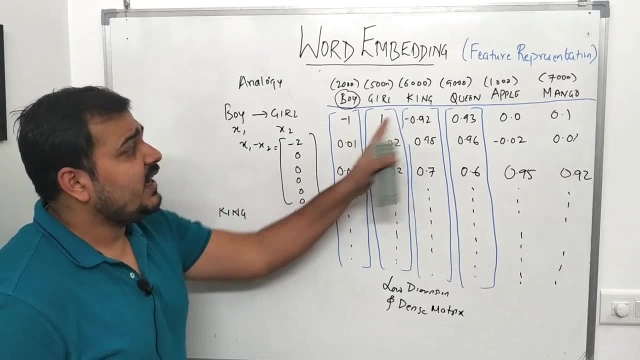 similarly, if I go and take King and Queen now, suppose, if I take King now, I want to find out which word is an analogy of King, right, which word is actually similar to King right now. if I take an example of King and Queen now here I will be actually finding out the difference and this: 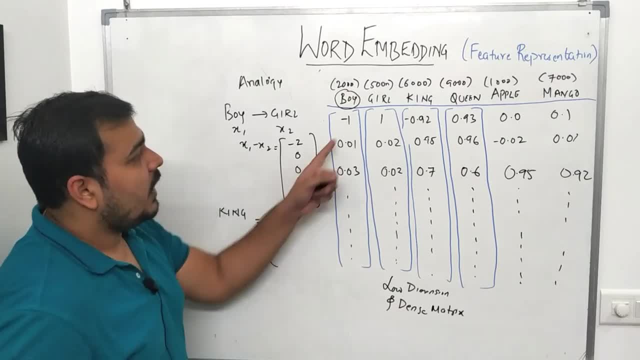 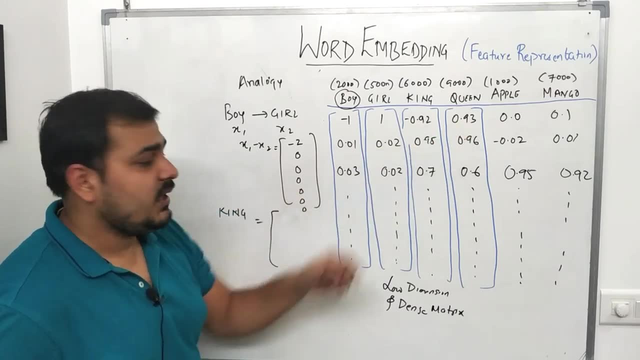 will also be somewhere near to minus 2, right. understand, this is minus 1 minus 2 minus 1 minus 1 in minus 2, right. if I do same thing: minus 0.92 minus 0.93, it will be somewhere approximately around minus 2, right, and the remaining all will be minus 1 minus 2, right and the remaining all will be. 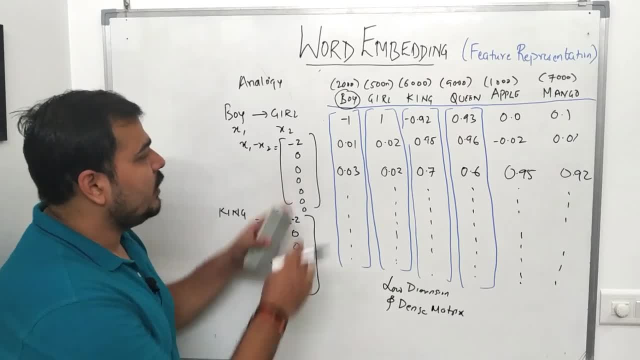 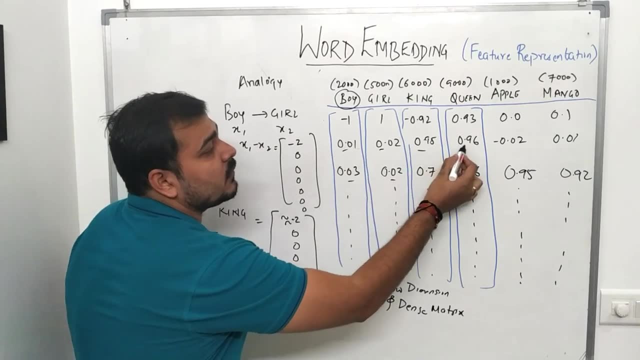 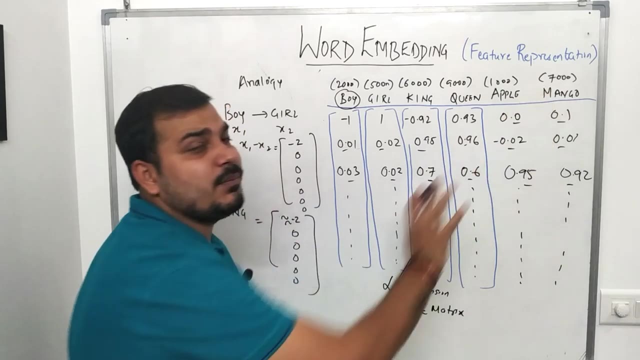 all the values will be 0, approximately equal to 0. understand this, guys. I'm not saying exactly 0, approximately equal to zeros, because these two values are almost similar. these two values are almost similar. right, these two values are almost similar because these two are similar words and. 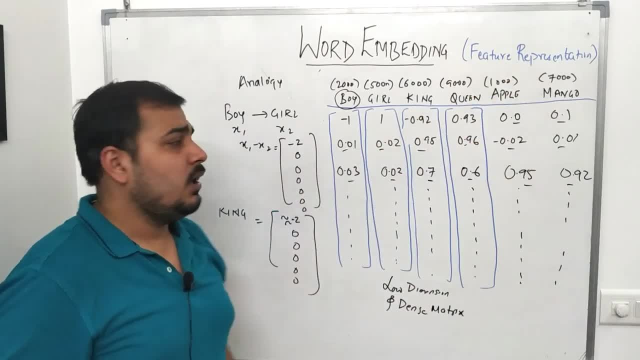 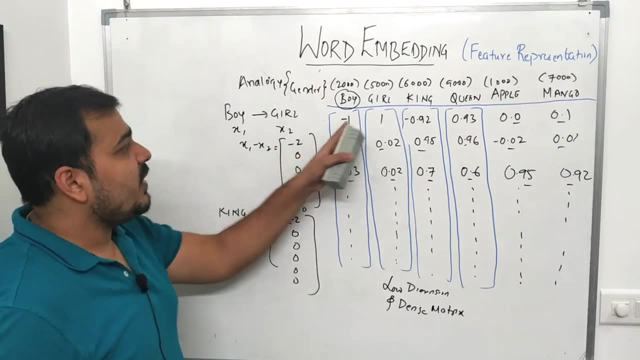 we are actually creating this vectorized representation based on feature. now this particular boy and all analog is considered from gender right now, based on gender, and based on this we can find out. suppose, if I am having an analogy saying that boy tends to girl, then what will King? 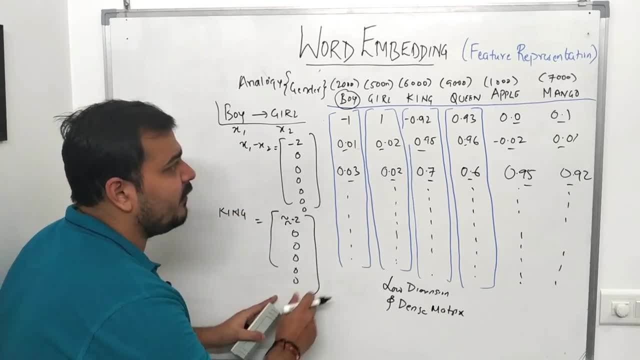 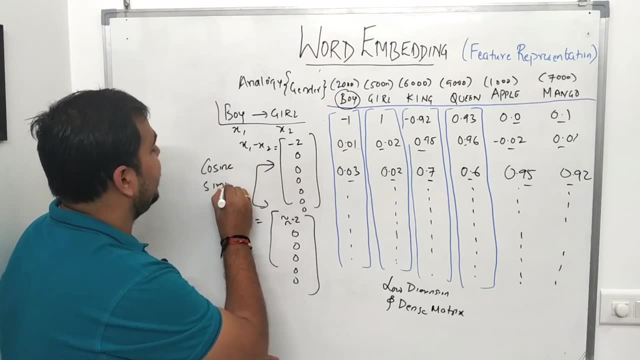 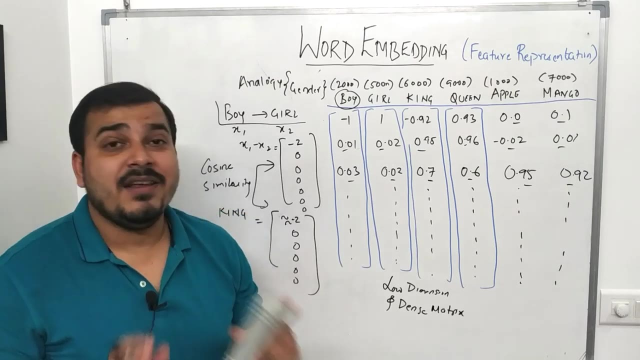 tends to. definitely, by seeing this difference, we will be getting this particular vectors with respect to Queen. now, if I try to find out the cosine similarity between them- cosine similarity, see guys, cosine similarity is heavily used in recommendation systems also. right, it is heavily, heavily used. okay, so if I use the cosine similarity, I will be able to find out that this distance is. 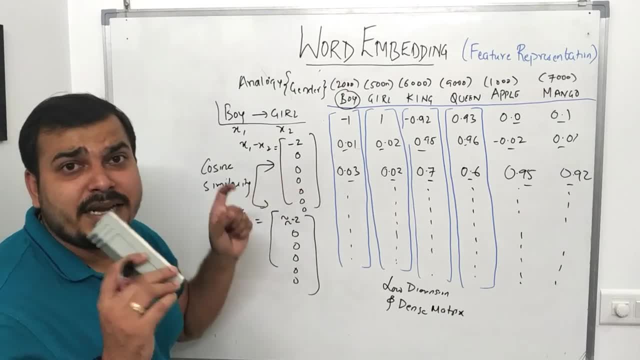 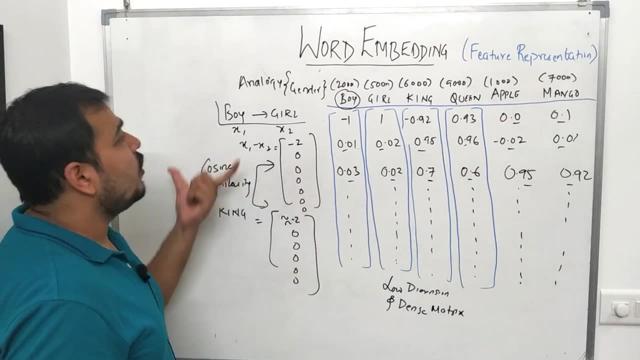 very, very less right this. when this distance is very, very less, then definitely my model can say that, okay, the most similar word to king is Queen, right? so like this, the whole representation is basically done, and this vectors play a very, very important role for doing this, because you will be. 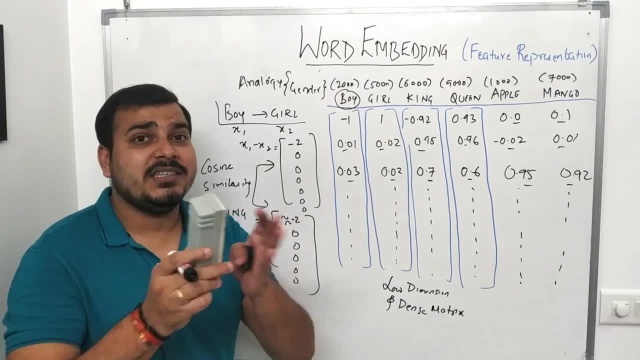 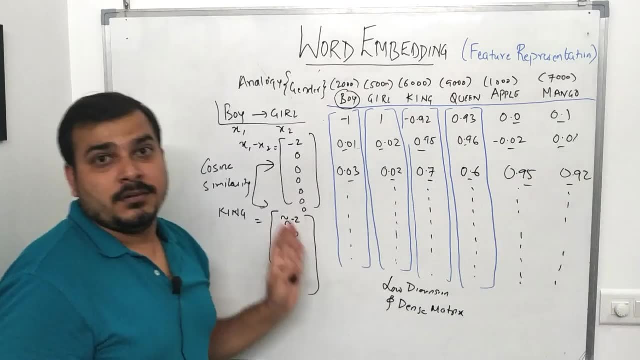 seeing that, guys, in the future, in the, in the upcoming classes, I'll be implementing lstm- recurrent neural Network- for some sentiment analysis. right at that time you will be seeing that I will be creating this embedding vectors. I'll be creating these vectors based on the, based on the text that I have. 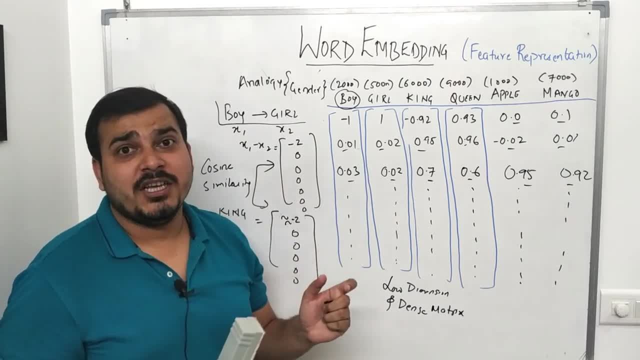 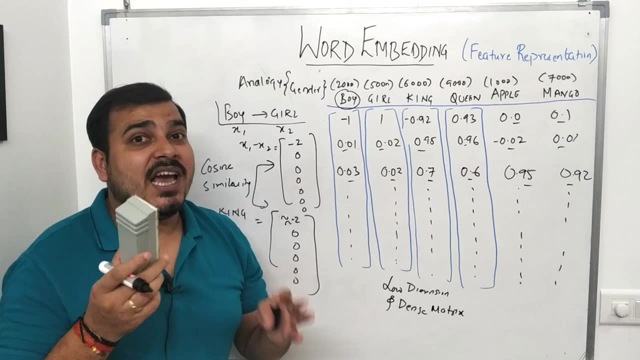 by using the same concept of one hot representation, and then finally, I will convert that one hot representation into this kind of featurized vector by using Keras. In Keras we have something called as embedding layer. You will love that. Probably tomorrow I will be uploading those videos. 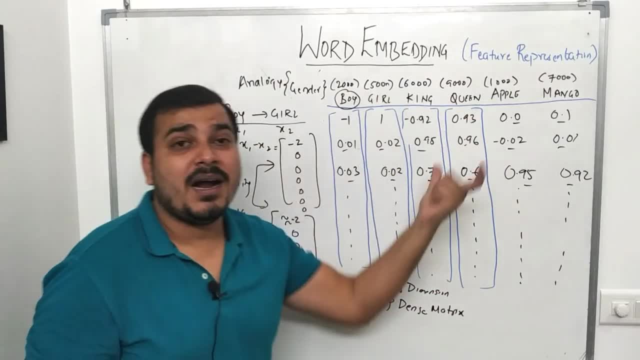 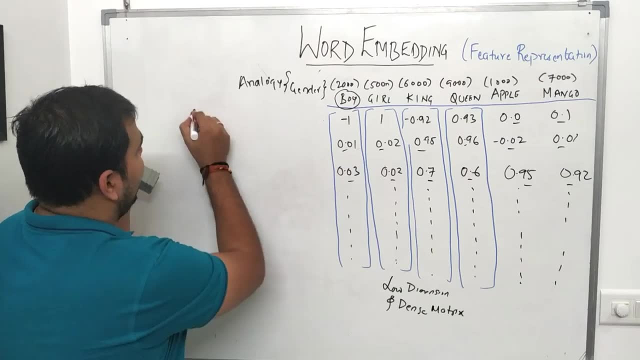 because you need to understand this thing. This is the intuition part of word embedding layers. Now, one more thing I want to basically represent. I am just going to rub this again. Now, I know that this is my 300 dimensions. right, You know that this is 300 dimensions. 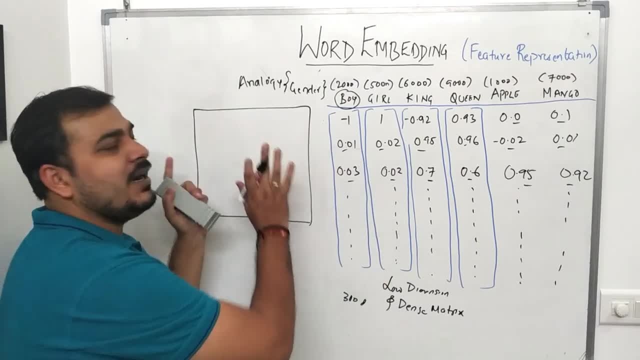 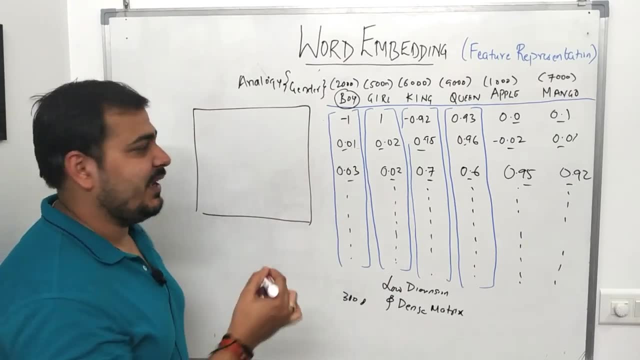 Now, if I convert this 300 dimensions into 2 dimensions, Suppose if I am modifying this 300 dimensions into 2 dimensions, At that time you will be seeing one more interesting thing. Suppose I have this point as king and queen, You will be seeing that. 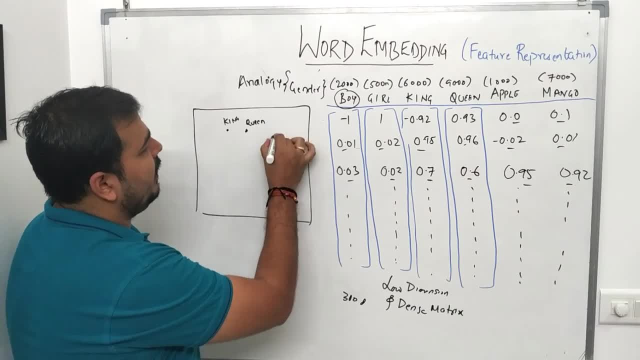 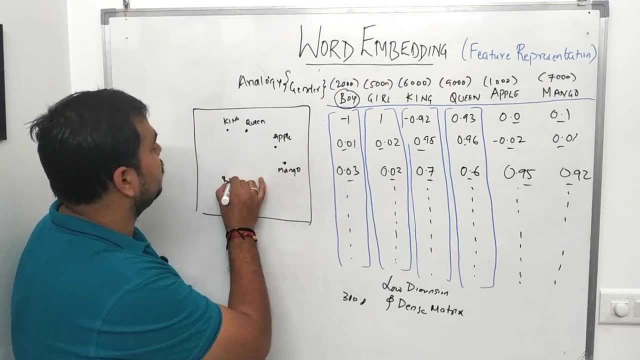 king and queen will be near. You will be seeing that apple and mango will be near. You will be seeing that boy and girl will be near, Or you will be also seeing man and woman will be near. So this kind of scenarios will be seen. 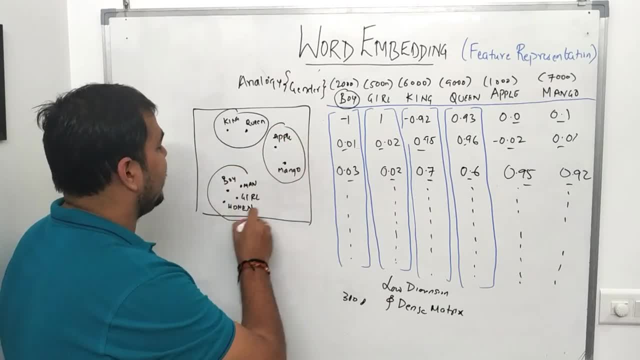 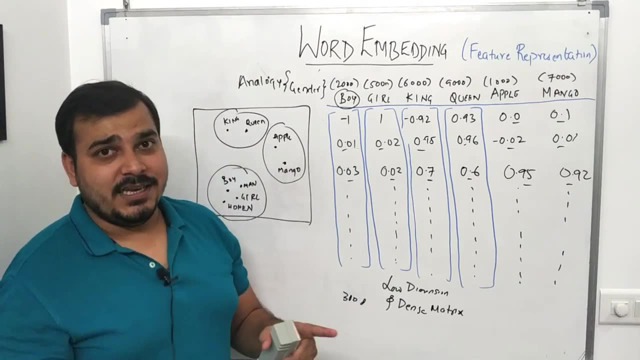 where you can actually group them into similarity, like when you are trying to convert this 300 dimensions into 2 dimensions. You know, by using some dimension reduction techniques, At that time you will be seeing that these all features will be very, very near to each other. So definitely. 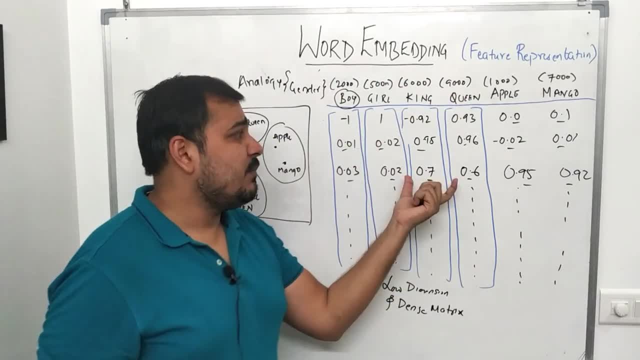 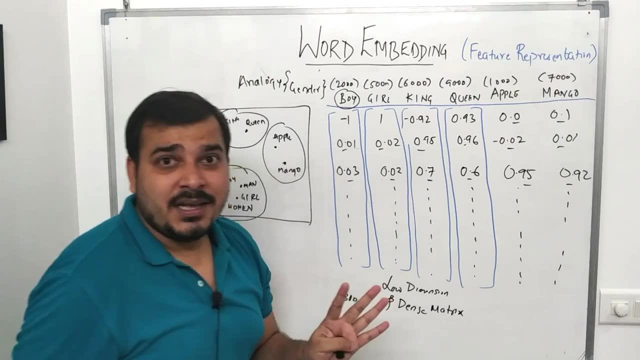 a word. embedding layer Helps you to find out the most similar vectors, because the vectors is created in that particular way only Right. So this is pretty much interesting to learn, guys, and word to wake is one of the embedding word embedding techniques. You have glove and you have. 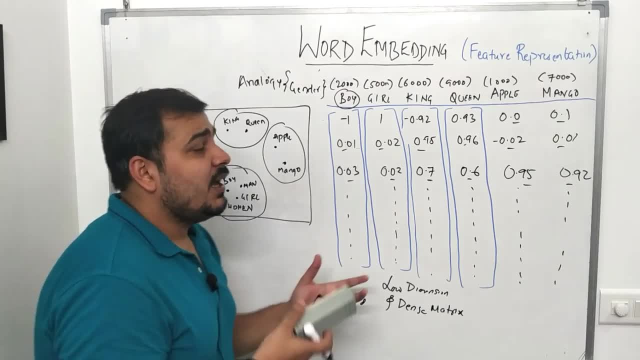 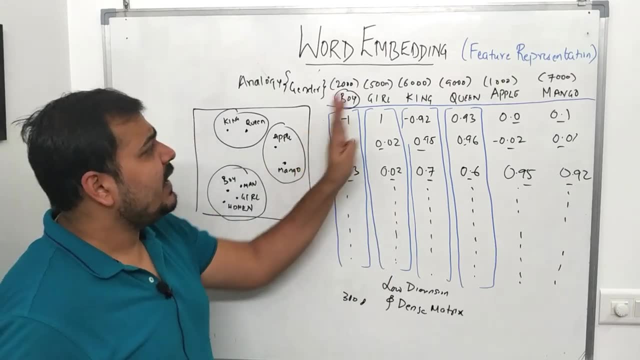 also libraries like gen, sim and all which will actually help you to get those vectorized kind of format of data. You know. you just have to pass the data, whatever data you have, and automatically it will be creating this kind of you know, vectors based on the number of dimensions.